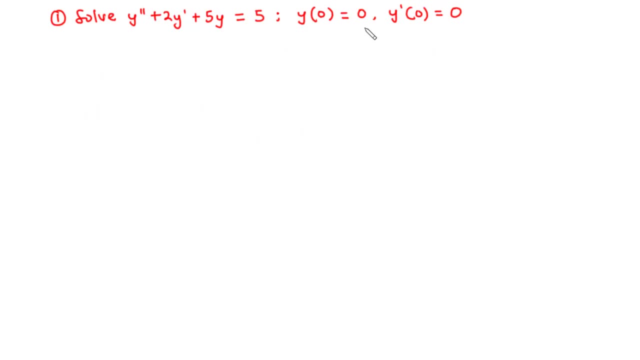 prime plus 5, y equals 5.. Given the initial conditions, y of 0 equals 0 and then y prime of 0 equals 0.. So let's try this together. So we have the second other linear differential equation: y prime prime plus 2, y prime plus 5, y. 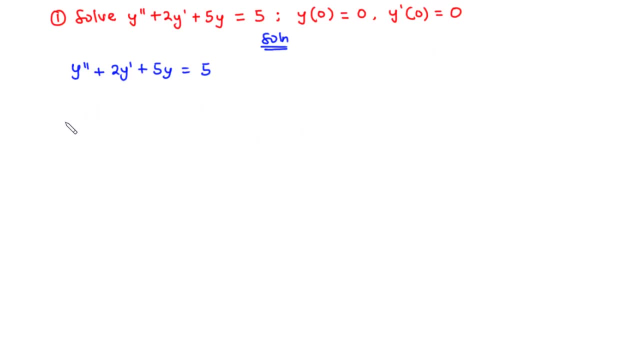 equals 5.. Now the first thing we are going to do is to take the Laplace transforms of both sides of the equation. So we have the Laplace transform of y prime prime plus 2, y prime plus 5. y equals the Laplace transform of 5.. 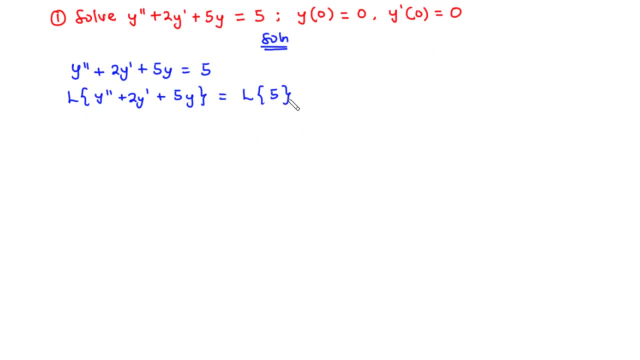 The next thing is we are going to use the linearity property of the Laplace transform to break down this transform into three transforms. So we are going to have the Laplace transform of y, prime, prime, plus we can pull out 2 because 2 is a constant. so plus 2. 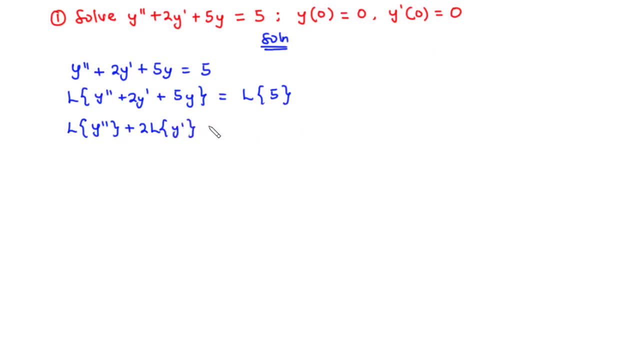 times the Laplace transform of y prime. plus we pull out 5 times the Laplace transform of y equals 5.. so 5 is also a constant here. so we pull out 5 times the Laplace transform of 1.. So at this point we have y prime prime and then y prime. here Now we know. 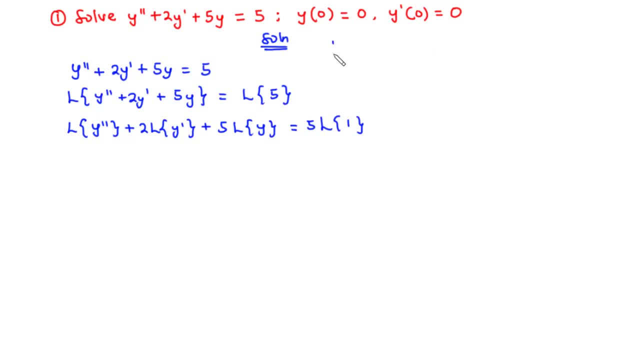 that the Laplace transform of higher derivatives is given by: we have the Laplace transform of f to the power n and that is given by s to the power n times. the Laplace transform of f minus s to the power n minus 1 times f, of 0 minus s to the power n minus 2 times f. prime of 0 minus dot, dot, dot, minus. 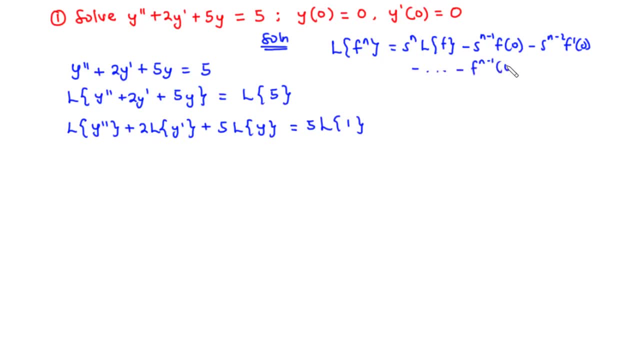 f to the power n minus 1 of 0.. This is the expression for the Laplace transform of higher derivatives. So we are going to apply this to find the Laplace transform of y prime prime as well as the Laplace transform of y prime. So for the Laplace transform of y prime prime, 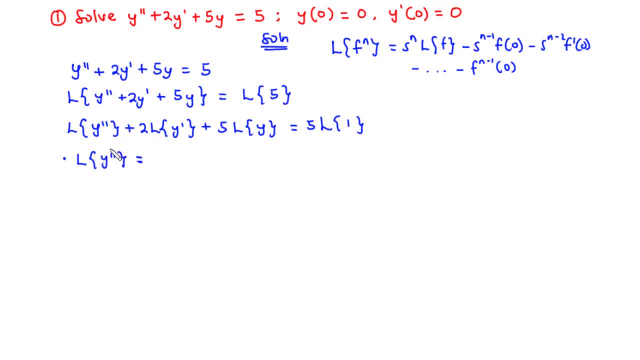 we have n to be 2, so that becomes s to the power 2 times the Laplace transform of of y, and then minus s to the power 2 minus 1 that is we have. I mean s to the power. 1 is the same as. 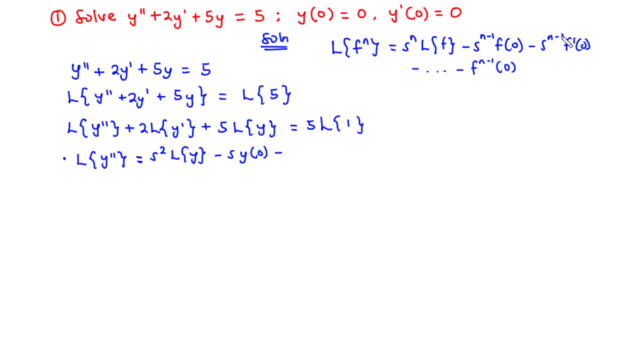 times y of 0 and then minus s to the power 2, minus 2, that is s to the power 0, ending on 0 number is to the power 0 is 1. therefore we have 1 times i prime of 0. now let's substitute the initial conditions, so we have y of. 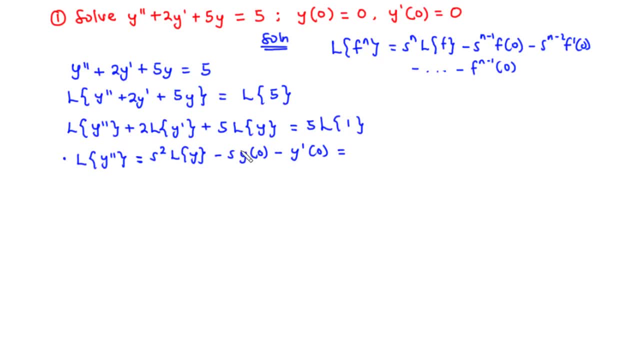 0 equals 0. we have y prime of 0 also equals 0, so these two terms becomes 0. and then we have s squared times the laplace transform of of y. now let's call this equation 1. also for the laplace transform of y prime, we have s to the power 1, so that is s times the laplace transform of. 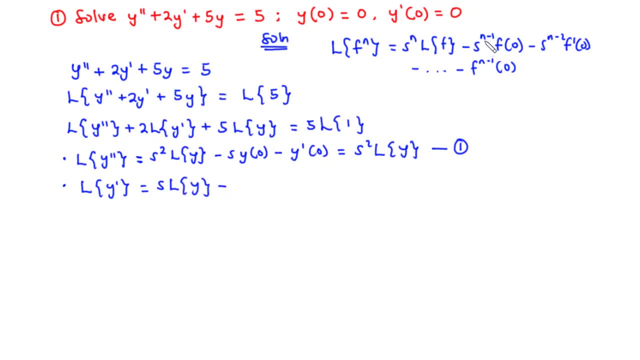 y minus s to the power 1 minus 1, which is exponent 0, so s to the power: 0 is 1, so we have 1 times y of 0, 0. y of 0 is 0, so finally this becomes s times the laplace transform of y. 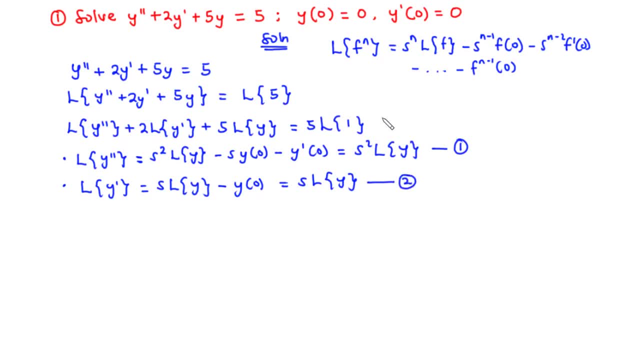 let's call this equation 2, and then we have the main laplace differential equation to be 3. so we are going to put equations, equations one and two, into equation 3. So for equation 3, we have the Laplace transform of Y, prime prime, which is S square times the. 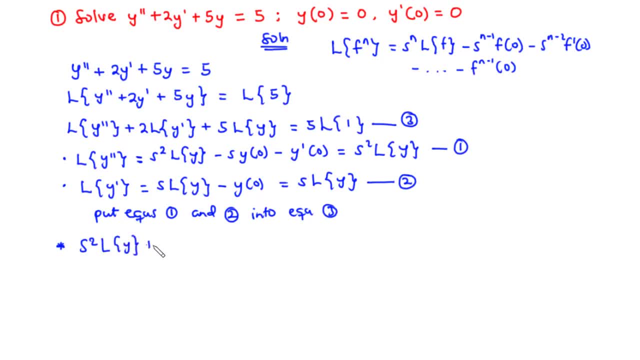 Laplace transform of Y plus 2 times the Laplace transform of Y prime, which is 2 times S times the Laplace transform of Y plus 5 times the Laplace transform of Y, equals 5.. Now the Laplace transform of 1 is given by 1 over S, So simply we are going to have 5 over S, 5 over S. Now. 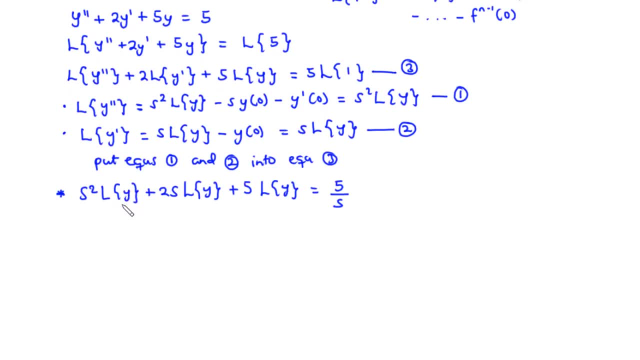 at this point we can factor out the Laplace transform of Y. So we are going to have s squared plus 2s plus 5 inside the bracket, so that on the outside we have the Laplace transform of y and that is equal to 5 divided by s. So the next thing: 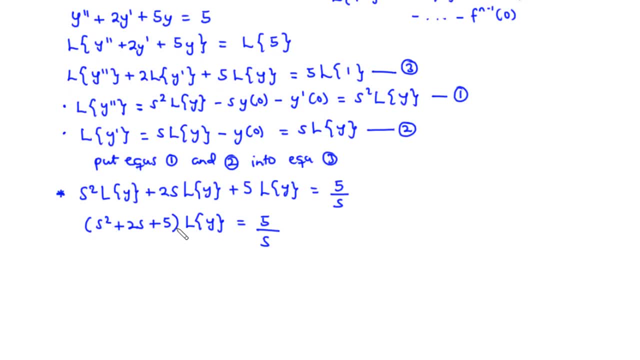 we are going to divide through by s squared plus 2s plus 5, and then that is dividing both sides of the equation by this term, and then thus we are going to have the Laplace transform of y to be equal to 5 divided by s, and then times s squared plus 2s plus 5.. So at this, 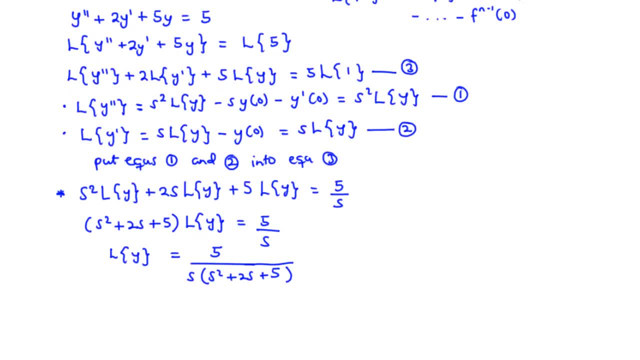 point. the next thing we are going to do is basically to find the inverse Laplace transform of this function. Now, at the denominator, we have s, which is a non-repeated linear factor, and then we have s squared plus 2s plus 5, which 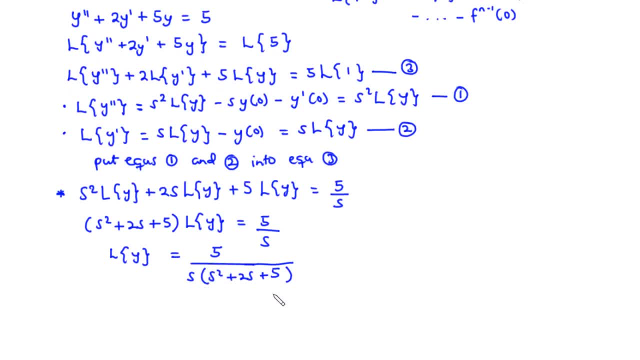 is a quadratic factor. Now we are going to see or verify if we can express this quadratic factor as the product of linear factors with real coefficients. So we have the coefficient of s squared to be 1, coefficient of the constant term to be 5.. 1 times 5 is 5.. We want to have 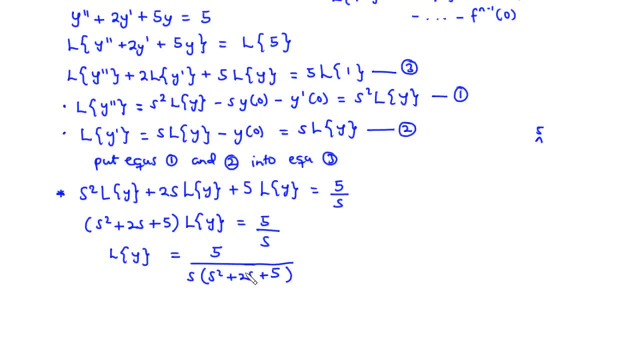 two numbers that when you multiply you have 5. however, when you add you have plus 2.. So i mean the factors of 5. we have 1 and then 5.. 1 times 5 is 5. however, 1 plus 5 is never. 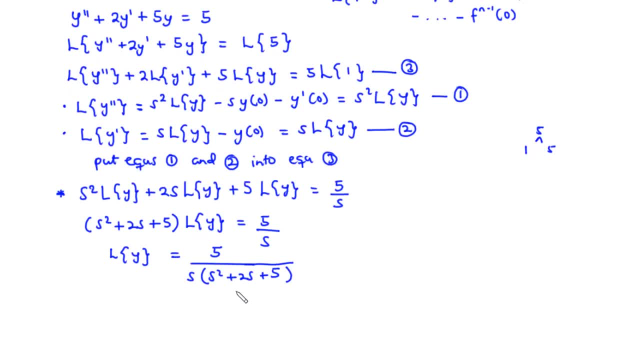 2, 1 minus 5 is never 2, and so on and so forth. So it means that we cannot express this quadratic factor as the product of linear factors. We are going to express s squared plus 2s plus 5.. So let's say we are going to express: 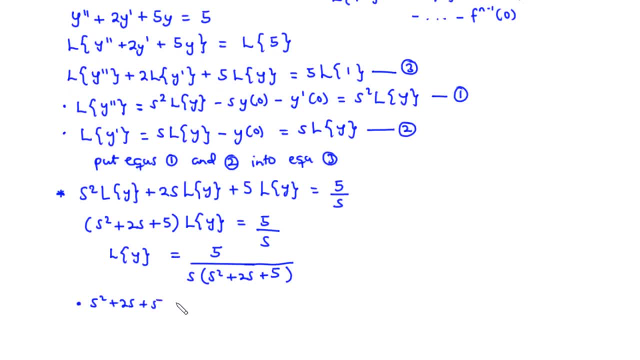 s squared plus 2s plus 5.. plus 5 in the form s minus alpha, or square plus beta, square, that is, completing the square. so so for s square plus 2s plus 5, doing the completing of square, we are going to have. 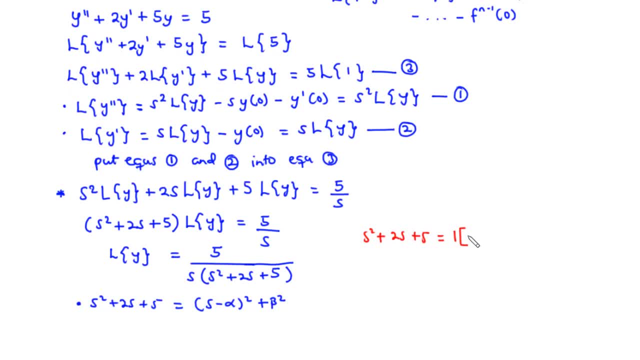 we are going to factor out the coefficient of s square, which is 1, so we have 1 outside and then s square plus 2s, plus now the coefficient of s here is 2, so we take that and then we take half of it, which is equal to 1, and then we square this value. so we are going to add. 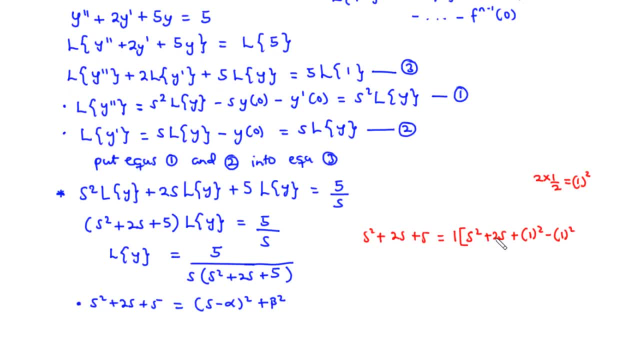 1 square, and then we subtract 1 square and then, lastly, we add 5.. so the next step, we are going to select s, and then this goes away. it goes away, and then we have s plus 1. this is a positive value, so plus 1, and then all square, and then this we have: 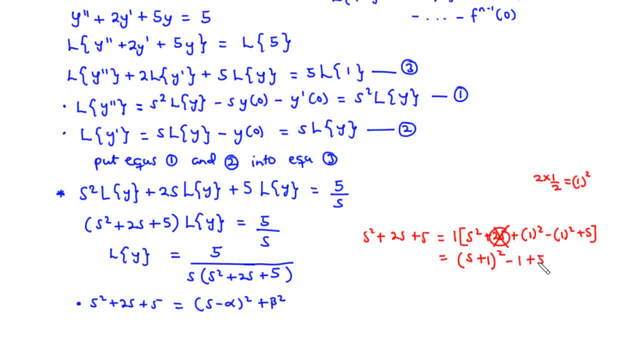 negative 1 square is 1 plus 5.. so this is s plus 1, or square plus 4, and then, since we want to represent this as beta square, we can basically have 2 square. so from this we say that alpha is equal to. comparing these two, alpha is equal to. 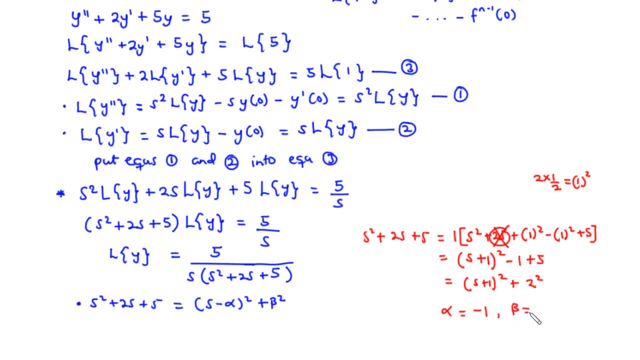 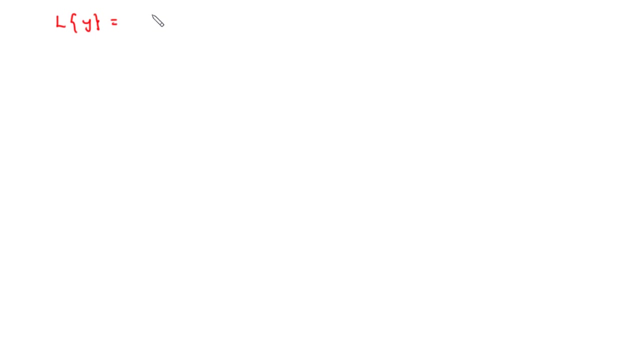 negative 1. and then we have beta equals 2.. so alpha equals negative 1, beta equals 2.. so we are going to decompose this rational function into the sum of simple rational functions. so we have the laplace transform of y, and that is equal to 5 divided by 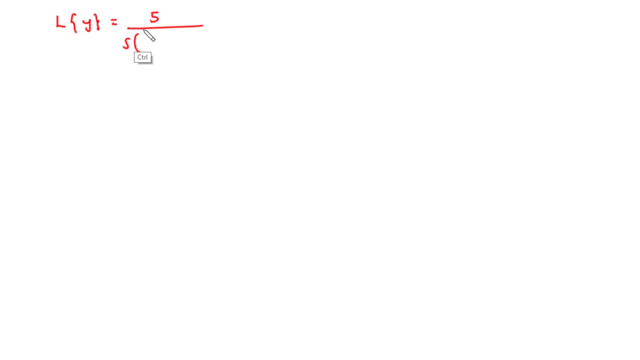 s. so we are going to represent, we are going to represent s squared plus 2, s plus 5 as s plus 1, or square plus 2 square, so that will be equal to. so first we have a quadratic factor, so we are going to express that as: 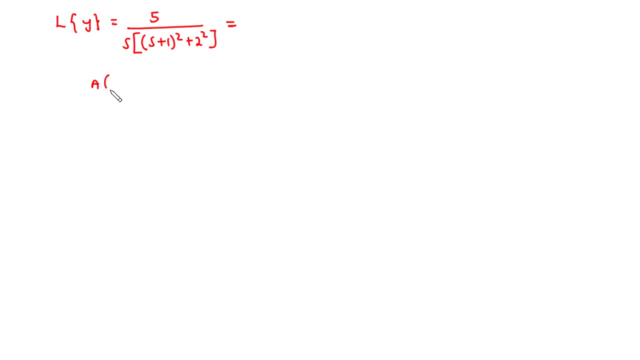 the exponent of the quadratic factor as a into brackets s minus alpha plus b, beta. now don't forget that we had alpha to be negative 1 and then beta to be 2.. so that's going to be s minus negative 1, so it becomes s plus 1 plus beta is 2, so 2 times b. so 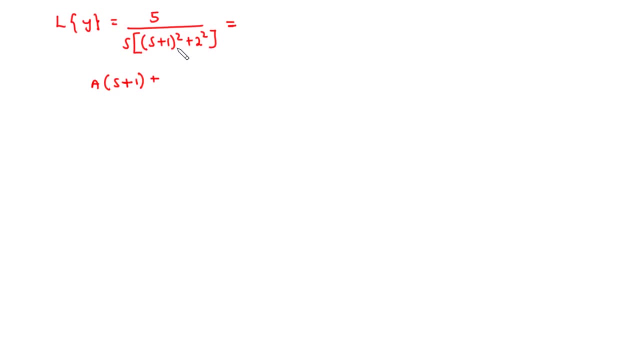 this is going to be the numerator of the quadratic factor, so a into brackets s plus 1. a into brackets s plus 1 plus 2. b, so divided by the quadratic factor, s plus 1, or square plus 2, square, and then plus c divided by the non-repeated linear factor, so c divided by s. now let's try to. 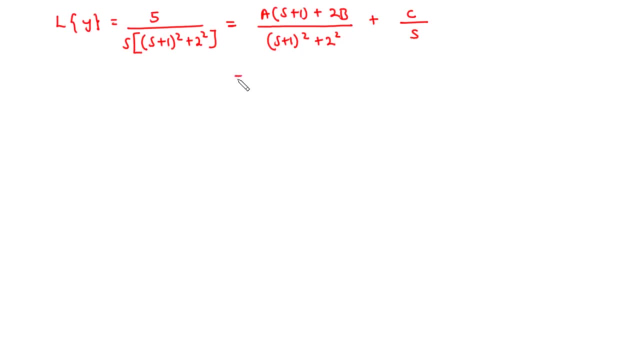 solve for a, b and then c. so first we are going to find the lcm that is going to be the product of these two. we have s on the outside and then s plus one, or squared plus 2. squared now this divided by that, we are going to be left with only s. so we have s, times a into brackets: s plus 1 plus 2 b. 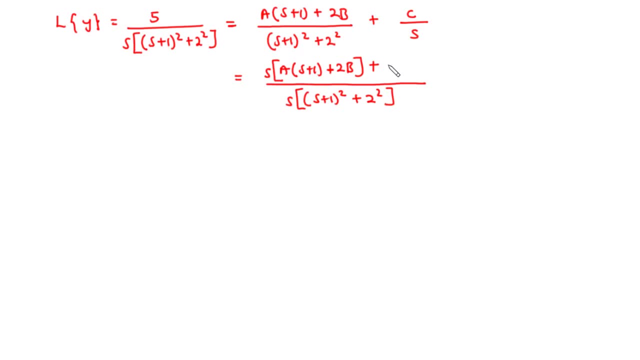 and then plus this, divided by that, you have s plus 1, all square, plus 2 square left. so you just multiply that by C. on the left hand side, we have 5 divided by. so, because the denominators are the same, we are basically going to work on the. 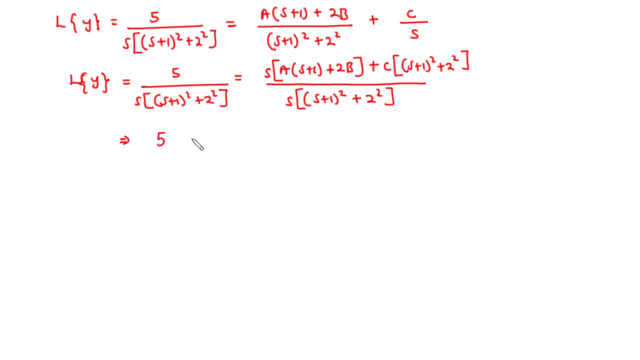 numerators. so we have 5. so if we put s equals 0, I mean this whole term goes to 0- we can find the value of C. so first let's try to find the value of C. you are going to put s equals 0. so for s equals 0, we have 5. on the left hand side that is equal to this. 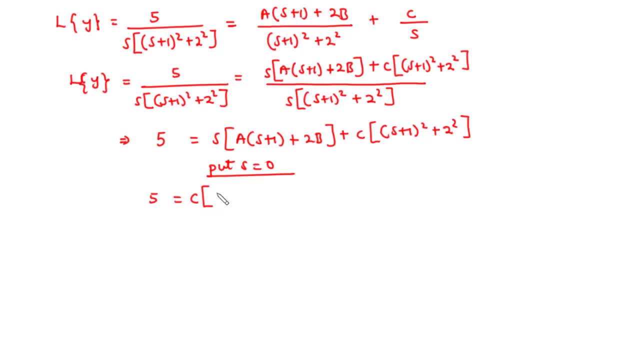 term goes to 0. we have C into brackets, 0 plus 1, all square, plus 2 square, which is 4. so this we comes: 5 equals. we have 1 square is this: 1 plus 4 is 5. so 5 C divided through by: 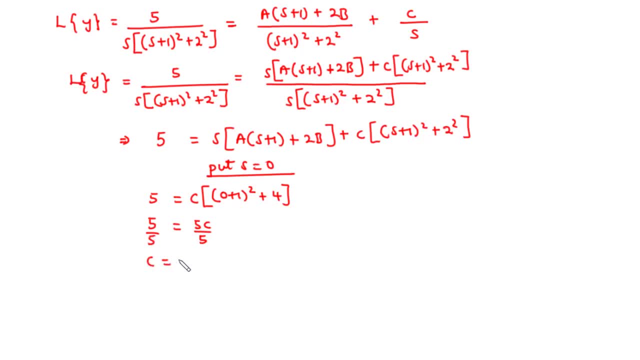 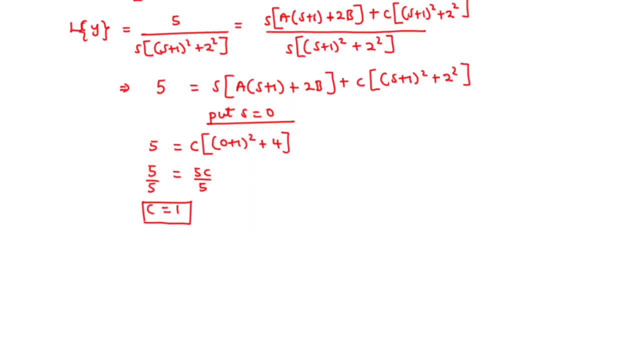 5, and then you have C to be equal to 1. so this is the value of C. now the next step. let's try to find either a or B. now, if we put s equals negative 1, a goes to 0. we can find the value of B using 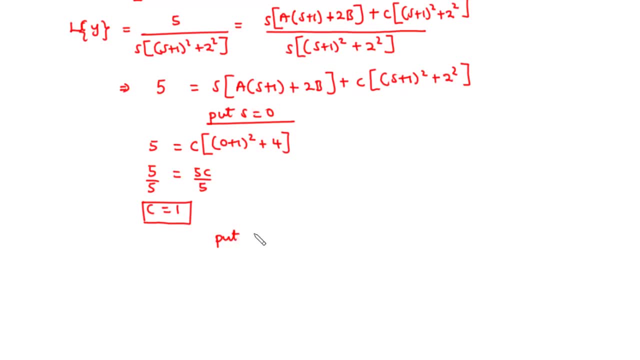 c equals 1. so next let's put: s equals negative 1. so if s is equals negative 1, on the left arm side we have 5. we have 5 equals negative 1 into brackets a into brackets negative 1 plus 1. so this goes to 0. so you should just clear this portion. 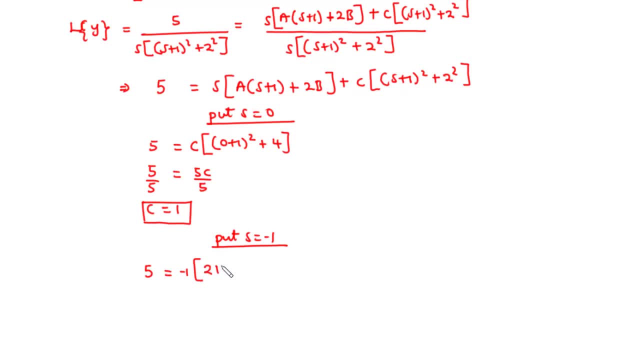 so we have plus 2b plus 2b plus 2b c into bracket negative 1 plus 1, all square, this is also 0, so let's just clear that. so plus 2 square, which is 4, so we have 5 equals negative 2b plus c. 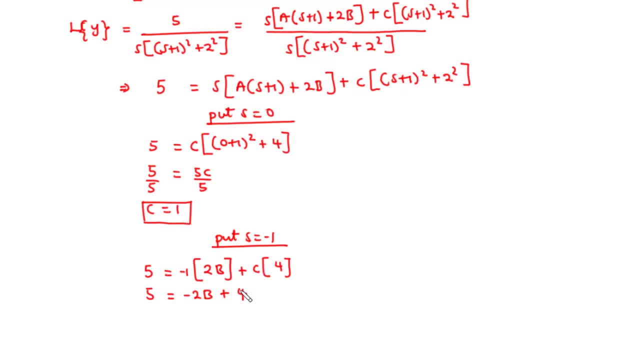 is 1, so 4 times 1 is 4. you transpose 4 to the left hand side, that becomes 5 minus 4 and that is equal to 1. so we have 1 equals negative 2b. we divide through by negative 2 and then we have the value of B to be negative 1 over 2. 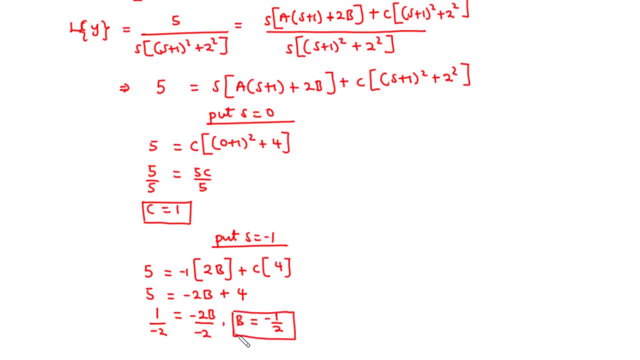 so this is the value of B. now let's try to find the value of a. so basically, to find the value of a, we are going to put s equals 1 and then we are going to make use of: I mean, c equals 1 and then b equals negative 1 over 2. so on the left hand, 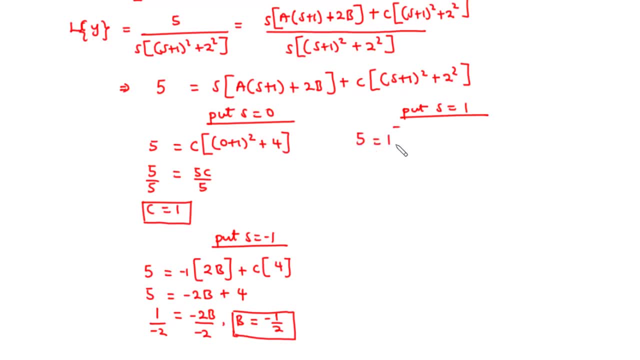 side we have 5 equals: s is 1. on the outside we have a into brackets: 1 plus 1, that is 2 plus 2b. now we have b to be negative, 1 over 2 plus c. on the outside c is 1. and then we have 1 plus 1, that is 2, so 2 square plus. 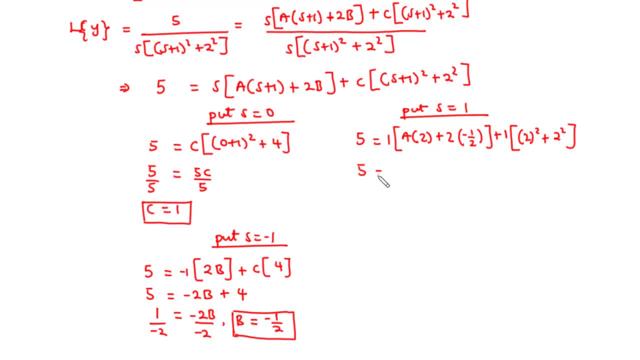 2 square 5 equals. this is 1. multiplying the whole of this, it's actually the same thing. so we have 2a minus 2 goes here once. 2 goes here once you are left with negative 1. so minus 1 and then plus 2 square is 4, 2 squares 4. so 4 plus 4 is 8. 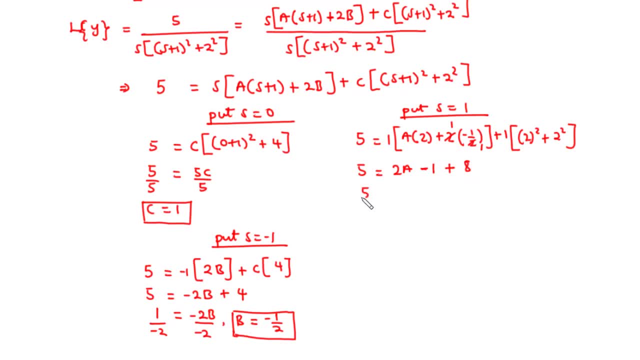 so negative 1 plus 8, that is plus 7. so we have 5 equals 2a plus 7. we transpose 7 to the left hand side, that becomes 5 minus 7, which is negative 2. so negative 2 equals 2a. we divide 3 by 2 by 2 and then we have a to. 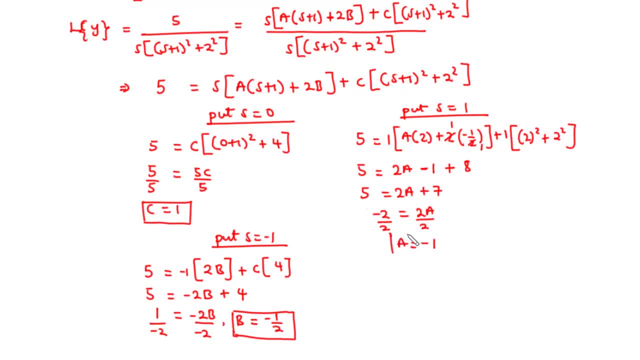 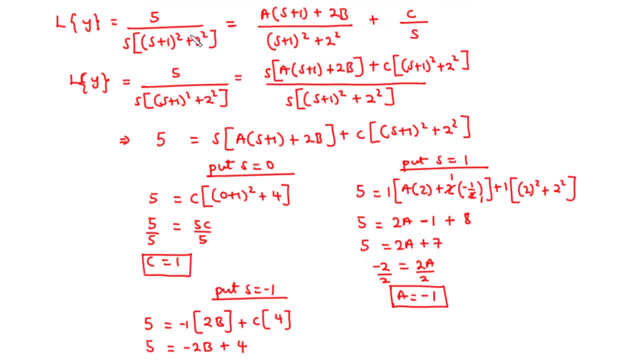 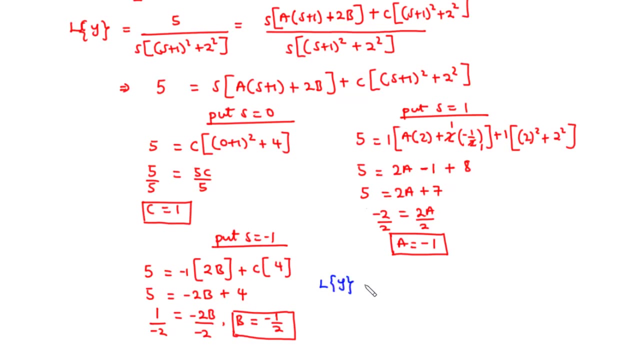 be negative 1, we have the value of a to be negative 1. so now the partial fraction decomposition of this rational function, which is given by the Laplace transform of y, can be expressed as we have a into bracket s plus 1 plus 2b. so a is negative 1, so negative 1 into bracket s plus 1. 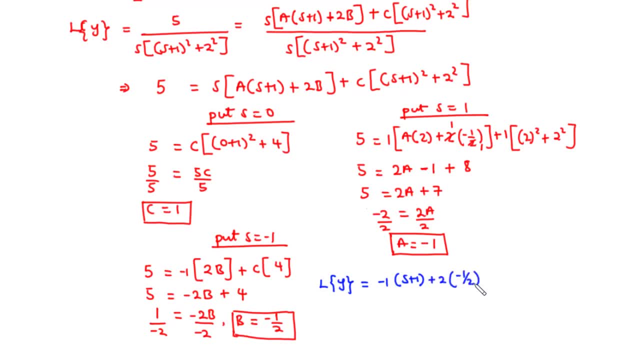 plus 2 times negative, 1 over 2, all divided by s plus 1, all square plus 2 square, and then plus c, so plus c is 1, so plus 1 over s. so this is the partial fraction decomposition of this complex rational function. now the next thing is to take: 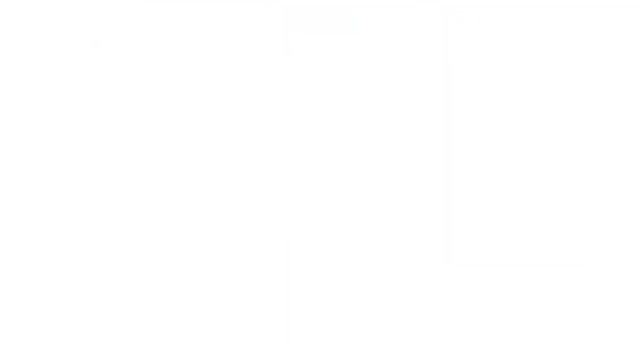 the inverse Laplace transform of this. so we have the Laplace transform of y decomposed into. we can express this fraction as: let's say, if you have a plus b, all over two, this can be expressed as a over two plus b over two. so we are also going to split this function, so this can be expressed as we. 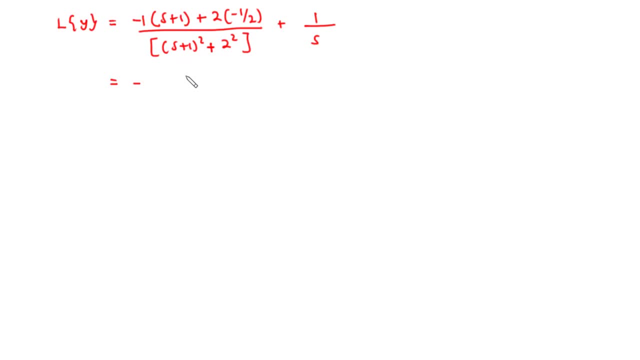 can have negative, negative one. so at the numerator we can have s plus one divided by s plus one all square, plus two square, and then minus two times one over two, also divided by s plus one all square plus two square, and then plus one over s. so this is the Laplace transform of y. 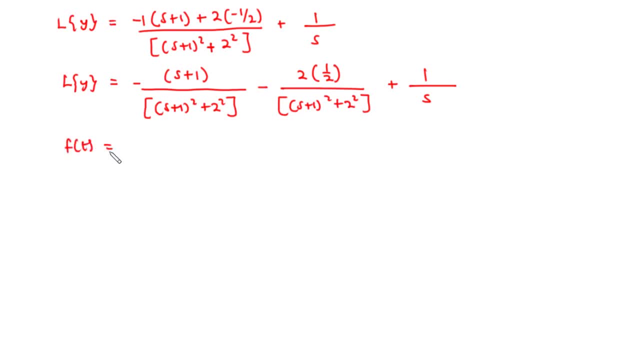 so we are going to take the inverse Laplace transform of y, so we have ft or f of t equals the inverse Laplace transform of of y, so that will be equal to the inverse Laplace transform of. I mean this whole thing. so let's say negative. 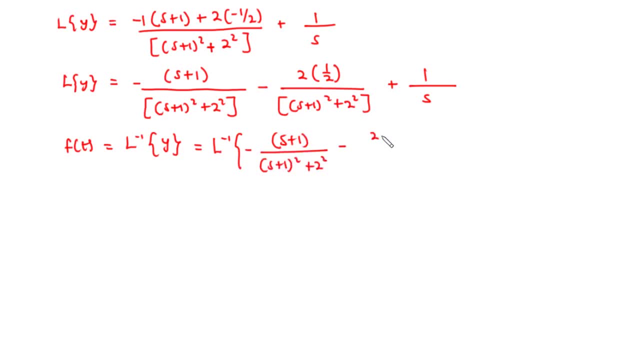 s plus one. so we are going to split this so that we have inverse Laplace transform of. so I mean this negative. because of this negative we are going to have, let's say, negative one or negative times, the inverse Laplace transform of s plus one all over s plus one all square plus two square. 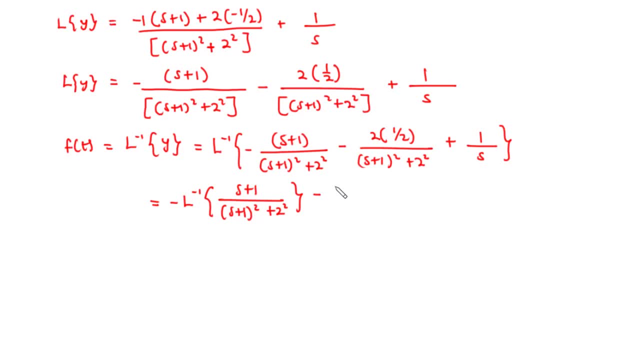 minus one over two, so one over two times the inverse Laplace transform of two divided by s plus one all square plus two square plus the inverse Laplace transform of one over s. now this transform here looks like a transform: s minus a over s minus a all square. 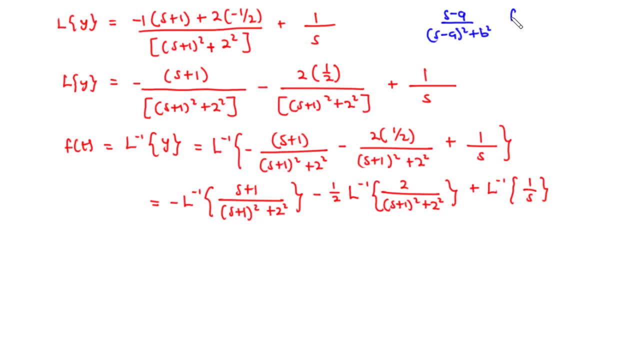 plus b squared, which is the transform of the function f of t, equals e to the power, a, t course, b, t, and so it means that, comparing these two transforms, we have a to be negative one, and then we have B to be 2. therefore, this corresponds to the inverse of this transform, corresponds to a function that 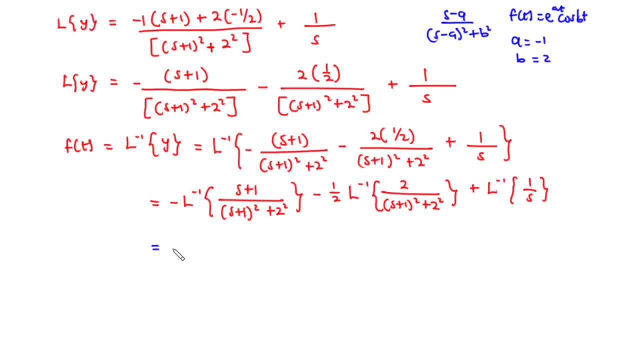 looks like this. so this is equal to: we have negative 1 times e to the power, negative 1 times t, so negative t and then cos 2t minus 1 over 2 times. this transform here also corresponds to b divided by s minus a r square plus b square, which also corresponds to the function f of t.